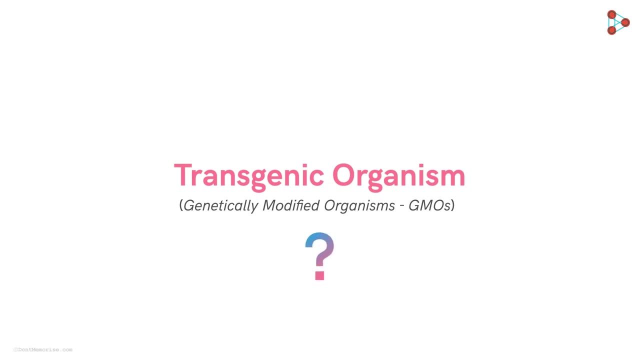 as GMOs. And what do we mean by transgenic or genetically modified organisms? An organism which contains DNA from another organism integrated into its genomic DNA is called transgenic organism. So will transgenic organisms be different from their original parental forms? Of course, 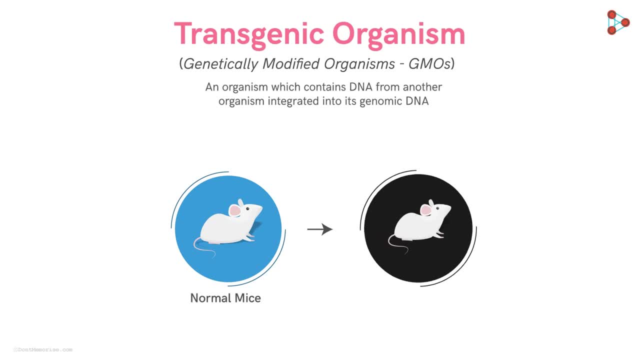 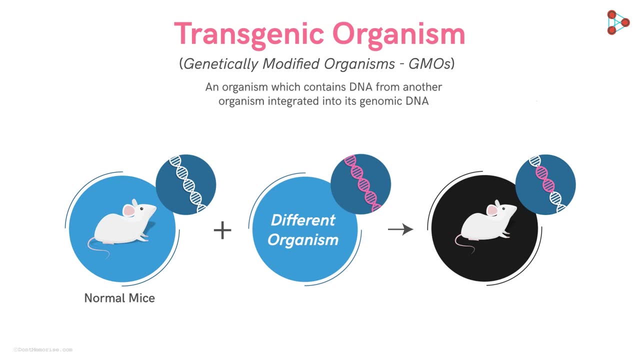 they will. A mice will not usually glow in the dark, but when we manipulate its genes, then the transgenic mice obtained shows the unusual ability to glow in the dark brightly. Let us get introduced to these examples individually. To begin with, we have the cotton plant named Bt cotton. 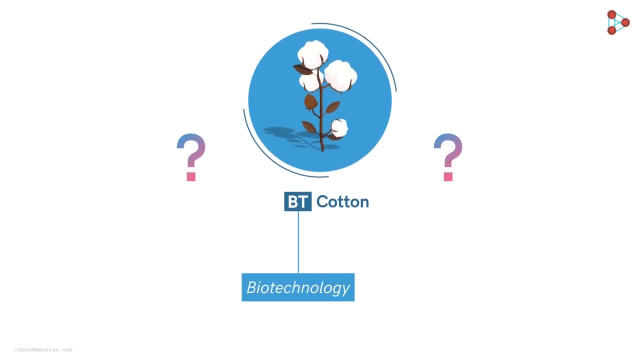 And what does this Bt mean? Does it stand for biotechnology? No, the prefix Bt stands for Bacillus thuringiensis, The bacteria which comes to the rescue of cotton plants. Have you come across the phrase? the enemy of my enemy is my friend. 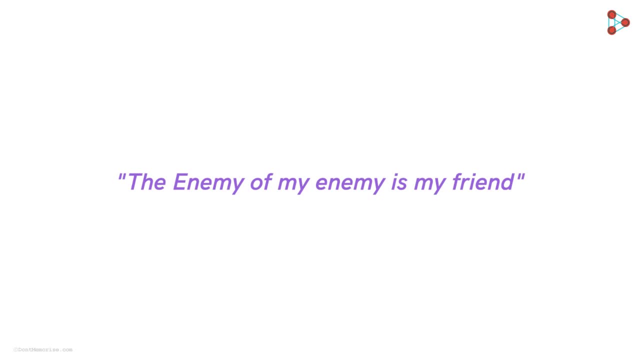 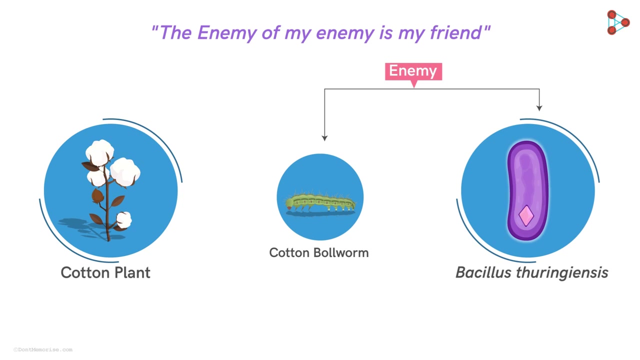 Well, that's exactly the case. we are going to look at Cotton plants have the biggest enemies in the form of insects And there are certain bacteria, like the Bacillus thuringiensis, which are like the enemies of these insects. They are actually capable of producing certain toxins that can kill these insects. 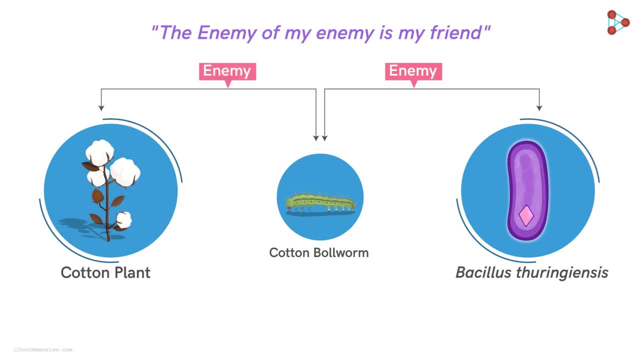 Does Bt For the cotton plant? their enemy's enemy, which is the bacterium, is like a friend, And this relation is exploited by genetic engineers to get cotton modified. Let us find out how. The first thing we need to know is about the protein and then about the gene which creates. 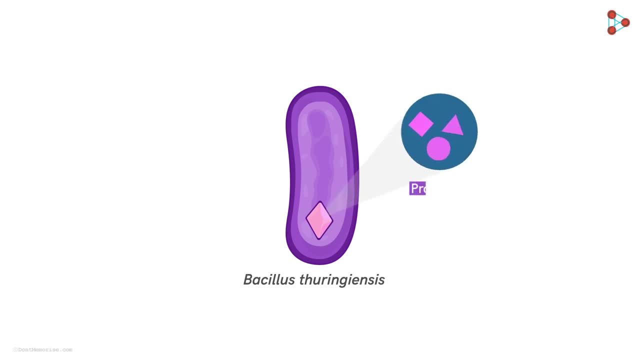 the magic. These bacteria produce certain proteins which are capable of killing various insects like cotton ball worms, beetles and others. So what is Bt? These proteins are also called toxins. The genes encoding the toxins is called cryogenes. And don't these toxins harm the bacterial cell?